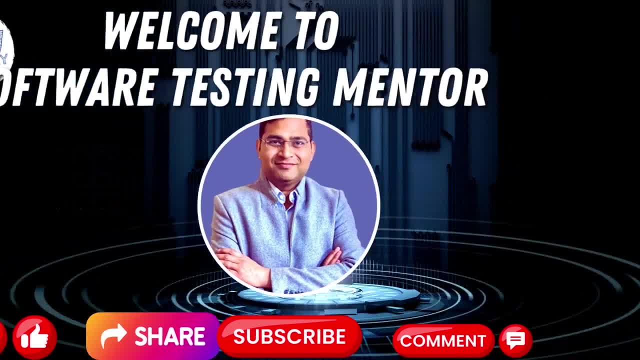 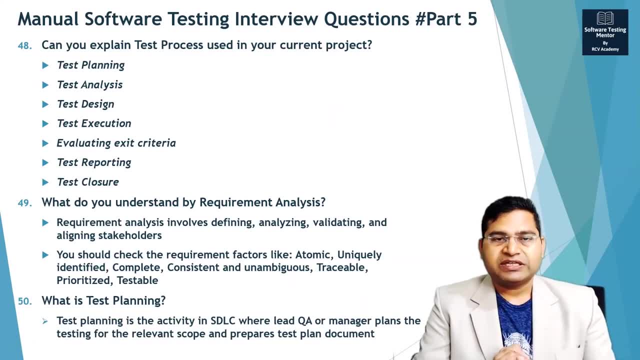 what is test planning? okay, now we have briefly touched on the test planning in question number 48 as well. so test planning is the activity. okay, test planning is an activity in the software development life cycle wherein the lead keyway or the test manager will go ahead and create a plan. 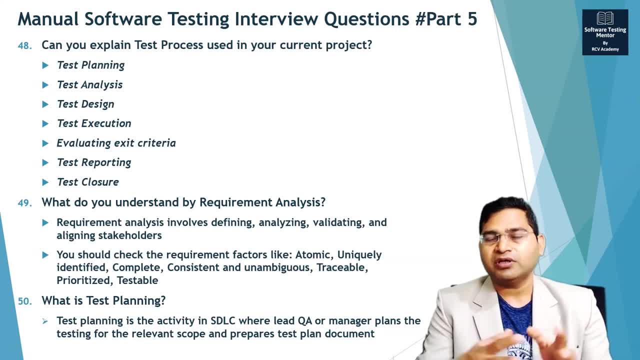 for testing. so if, say, for example, your release is for three months or six months or a year, a test plan document will be created which will have the details of what will be tested, what is in scope, what will be tested, what will not be tested, what are the timelines when the testing will start and 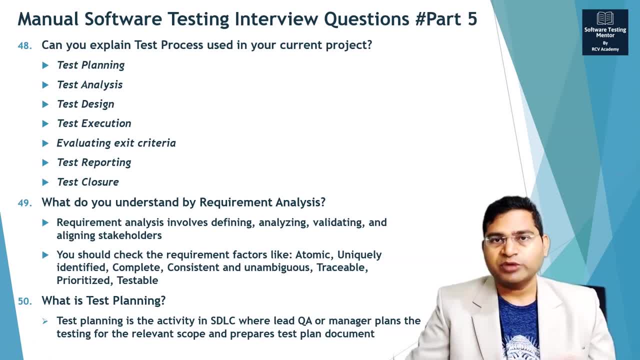 finish. who will be testing all of this? okay, how many team members will be required then? entry and exit criteria, all of those details, as we have already covered in one of the previous interview question video, which is, I think, part three or four, as per the test plan template, all. 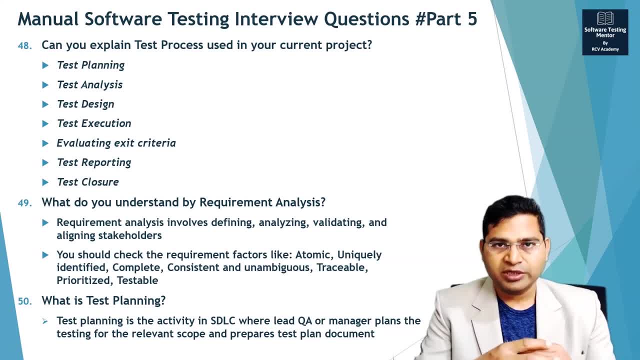 of that information will be filled in that word document or test plan document. okay, mostly it's a word document and that is what happens in the test planning. so analyzing what needs to be done and then planning the whole testing across for that particular release is test planning. now. 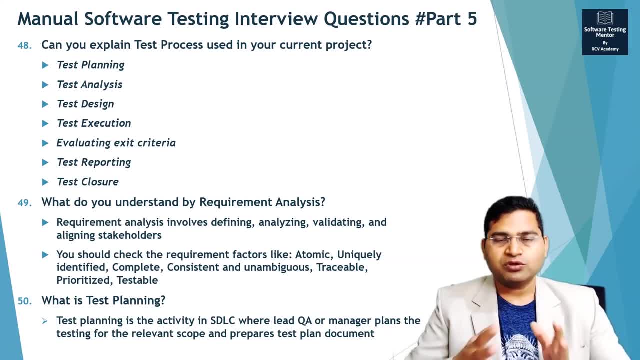 test planning also happens within the sprints. okay, so if you're following agile software development approach, so test planning is a part of the test planning process and testing is a part of the test planning process, so test planning will also be applicable within the sprint, which is two to. 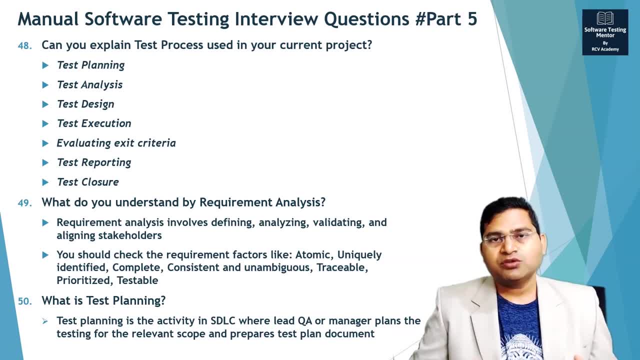 four week cycle wherein say, for example, for two weeks you have been allocated, or, or in the sprint planning, there will be some stories that are part of that particular sprint. now developers will develop it, testers will write test cases and finally test it right. so before you go ahead and 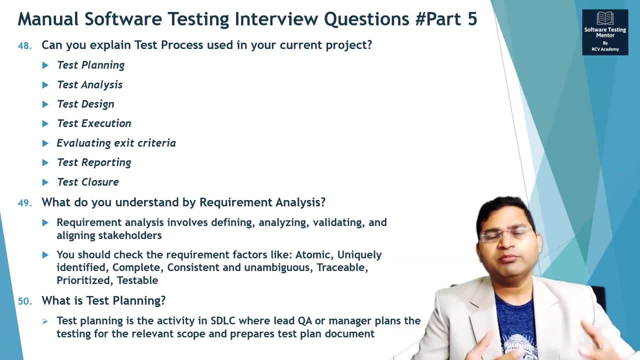 write test cases. you need some sort of planning, or very minimal it's. it's not massive planning. you don't create massive document in those two weeks, right, it's just high level planning and discussion with the team, testing team and even including developers. so basically, what is in? 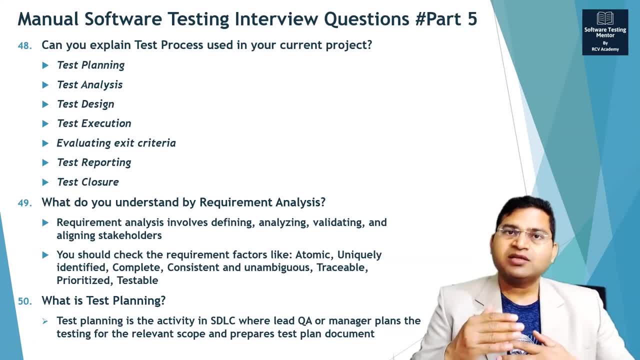 scope of, as as these stories, what will be tested, what won't be tested as part of this scope- the two week scope or four week scope, whatever the sprint duration is, and what will be the exit criteria? what will be the definition of done when we say testing is is done right or what will be?